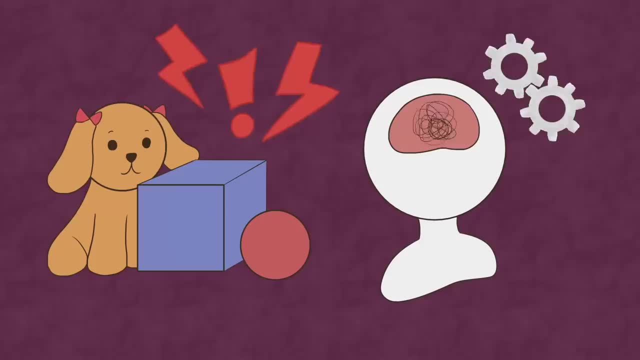 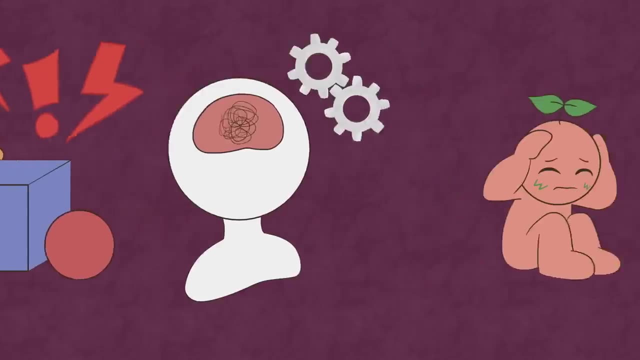 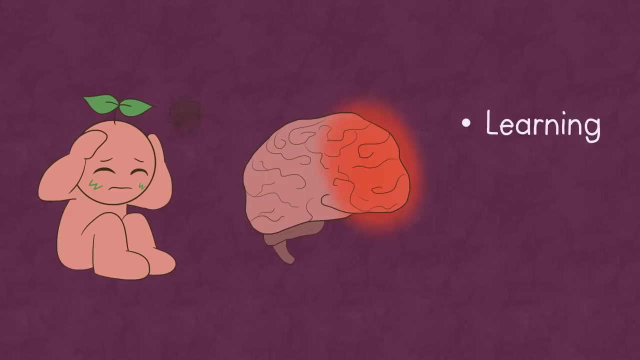 In truth, the reason might lie within your childhood. Research shows that those who suffered significant trauma at a young age cannot correctly consider risk as adults. Experiencing extreme stress during early development has been shown to cause changes in the frontal areas of the brain associated with learning. 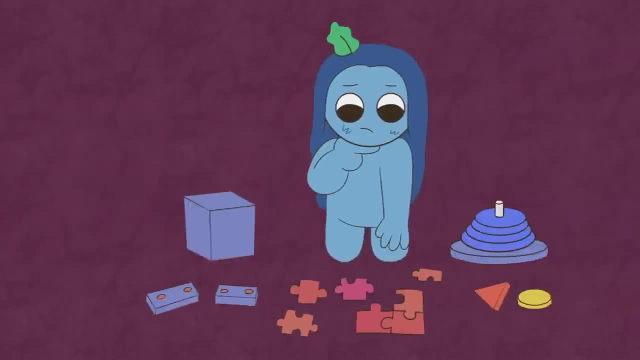 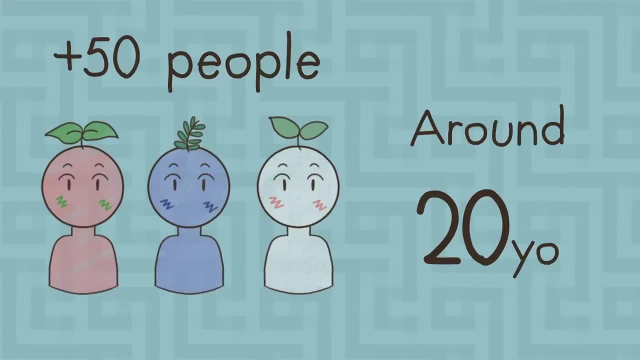 decision-making and memory, causing interference with the formation of the connections and networks that support thinking and learning. A study with over 50 people around the age of 20, and over 50 people around the age of 20, found that those who had experienced extreme stress. 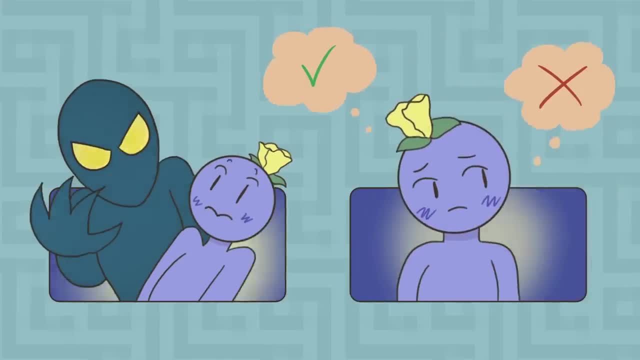 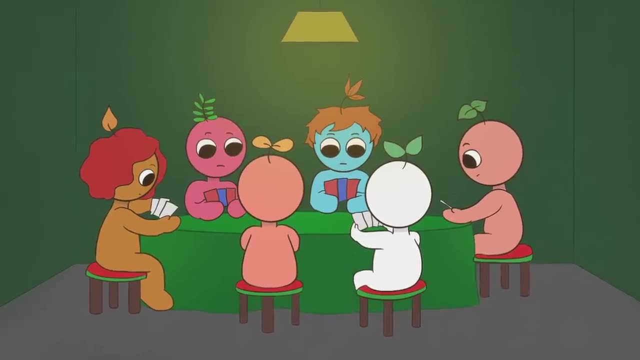 as kids were hampered in their ability to make good decisions as grownups. The study involved adults engaging in gambling situations designed to assess their response to risk-taking, reward and punishment. The results showed that the people who did not have stressful childhoods tended. 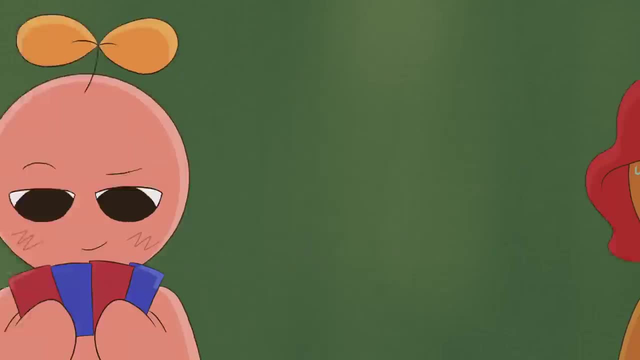 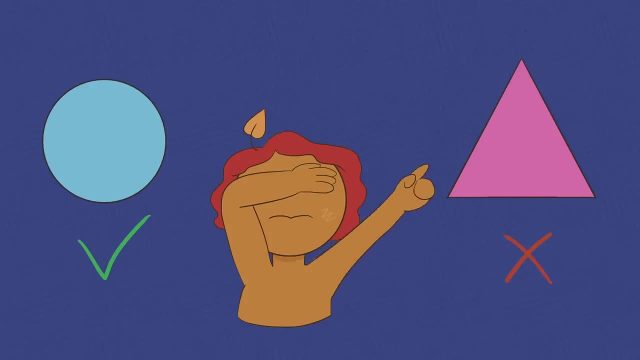 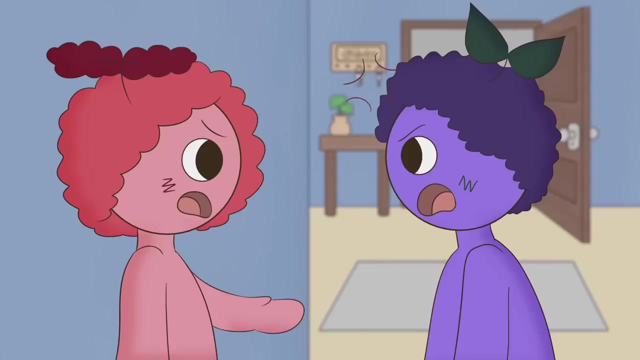 to pay attention to the clues and gamble wisely. Those who had suffered severe trauma did not. They would, for instance, choose the shape they had been warned against and make a mistake repeatedly. Number two: Interaction with others in relationships. Loving is hard, but it can be even harder. 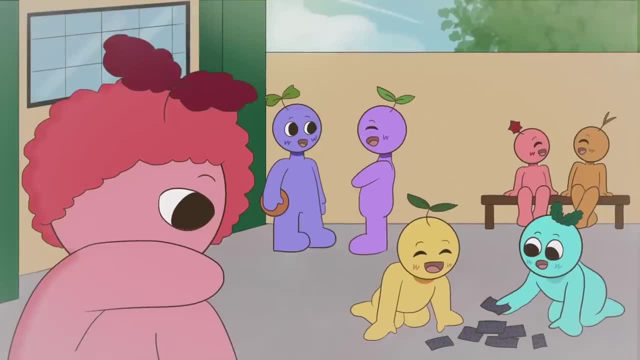 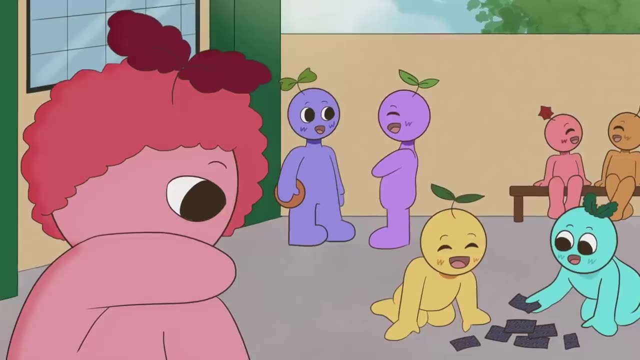 if you've suffered from distressing memories in your childhood, If you've experienced trauma during the first years of your life, then the odds are you might look at and experience adult relationships in a certain way. Perhaps you don't feel safe all the time. 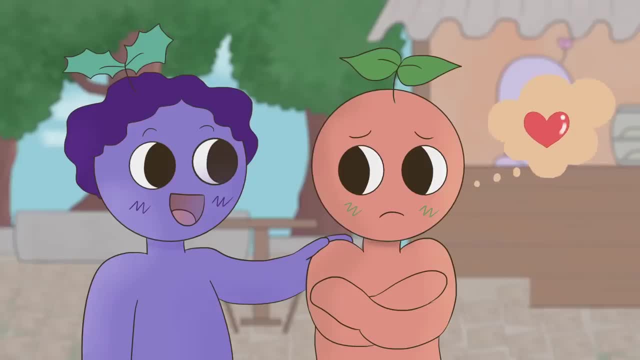 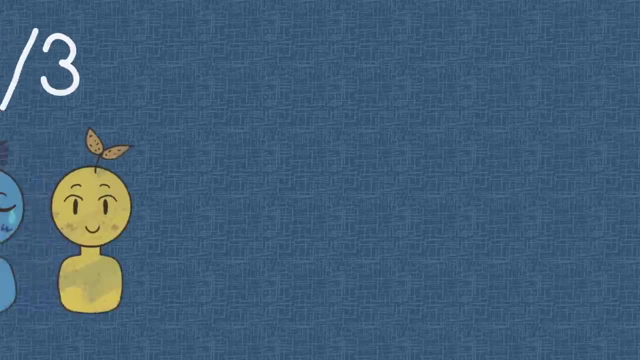 even when you're in a healthy relationship. Perhaps you hesitate to open your heart to anyone. If you're feeling this way or experiencing relationship challenges, know that you're not alone. In the United States, more than half of the population, more than two-thirds of children 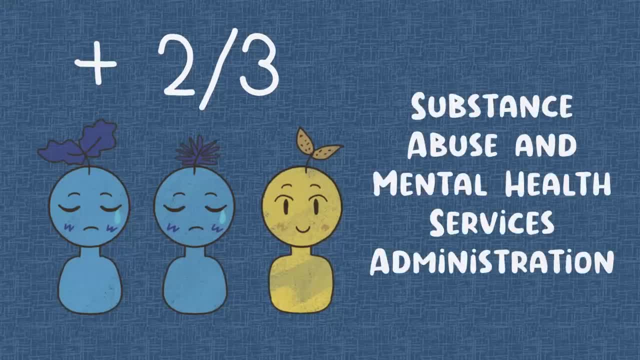 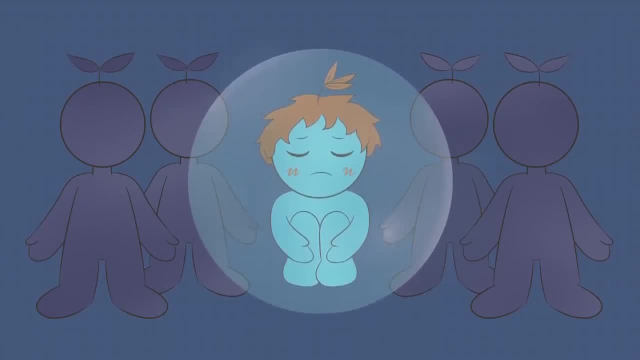 have experienced some form of trauma, according to the Substance Abuse and Mental Health Services Administration, And there's a myriad of ways that childhood trauma could impact the way you experience adult relationships In early childhood. secure attachment develops within loving, nurturing and stable relationships. 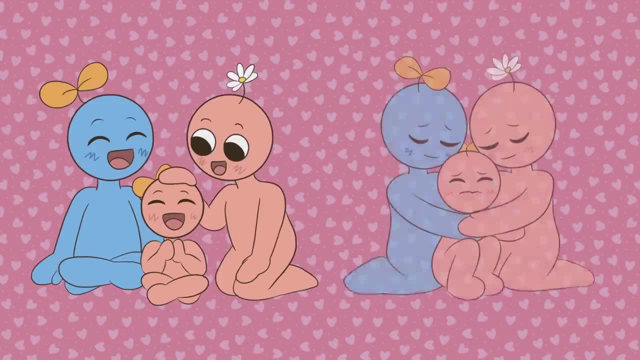 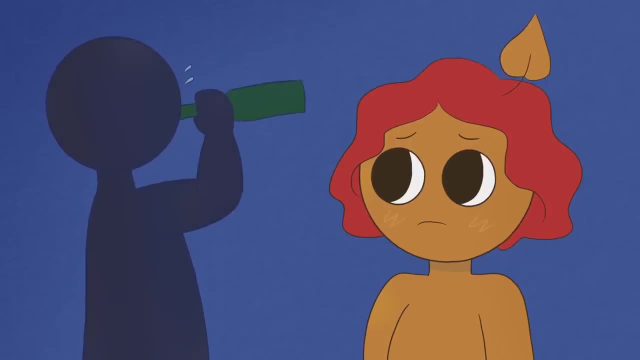 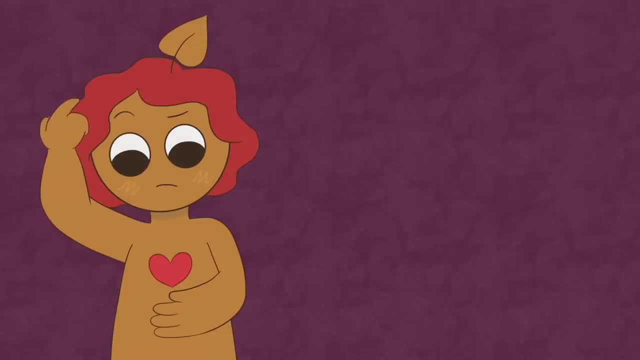 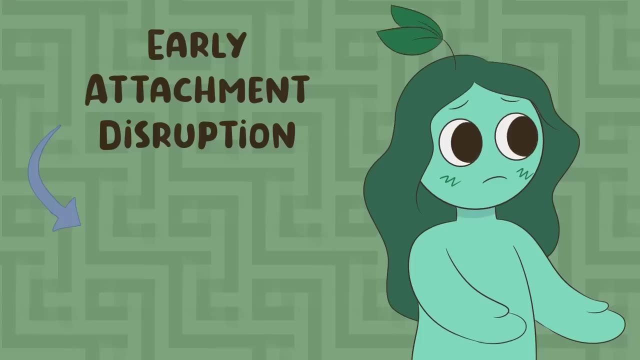 your ability to deal with it. your ability to deal with it, your ability to form such attachments is disrupted, resulting in attachment injury, trust issues and even mental health conditions. Early attachment disruption can cause an internal attachment disorder. later This mirrors the emotional injuries.